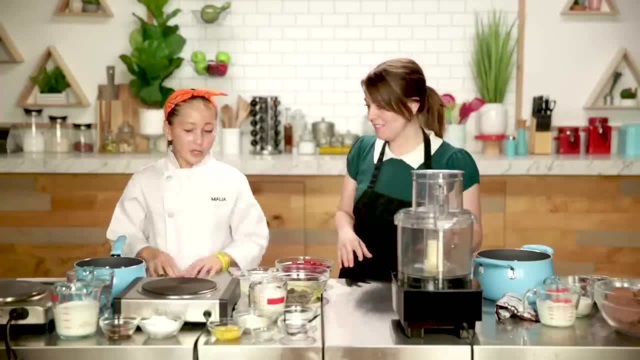 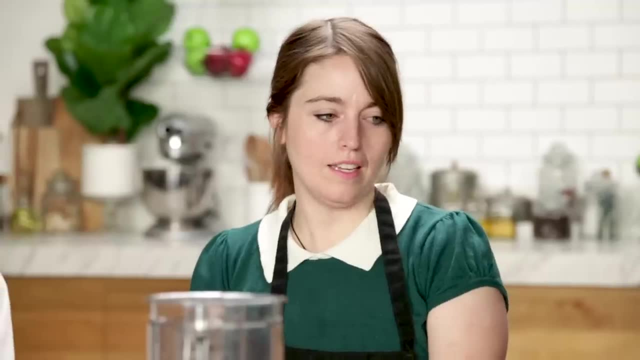 I have a black apron, But yeah. so what are you making? So I'm making a chocolate souffle with a raspberry coulis and a dollop of whipped cream. I am making a chocolate, dark chocolate caramel tart with a chocolate cookie crust. 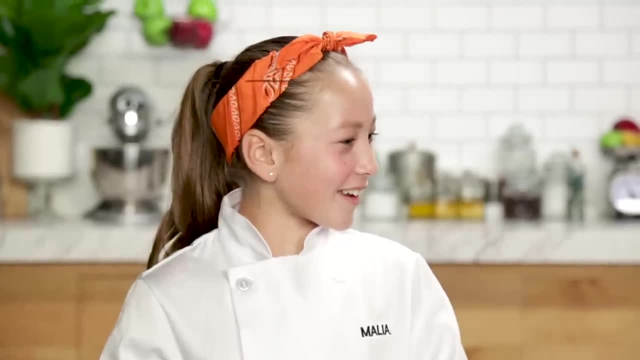 and a little sea salt to go on the top. That's fancy. Thank you, Okay. well, before we begin, let's wish each other good luck. Do you want to shake or do you want to Hug? Oh my gosh. 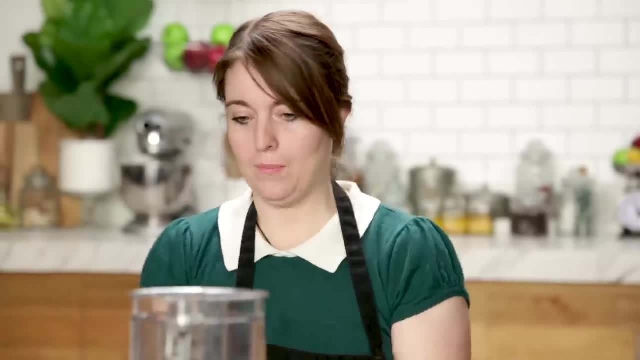 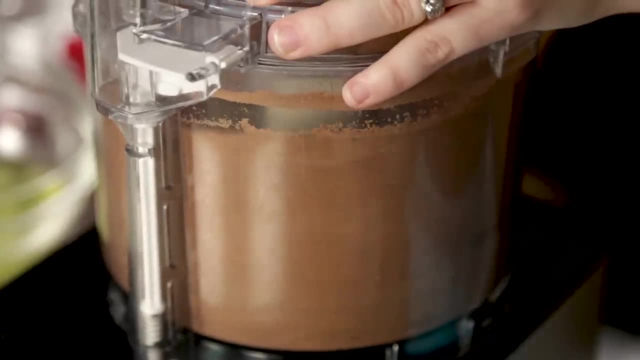 Okay, let's hug. Good luck, You're awesome. Okay, good luck. My first step is I'm going to make my crust. I'm going to food process these cookies so that they get ground down like a sand texture to make my tart crust. 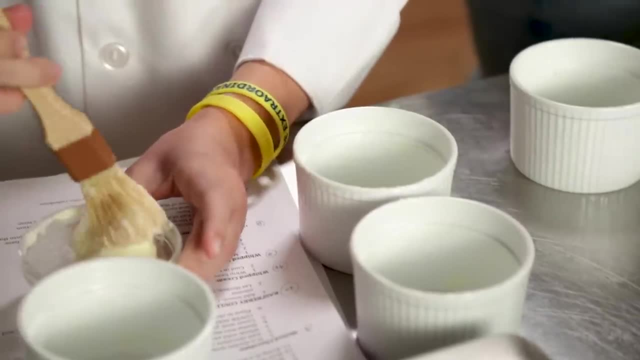 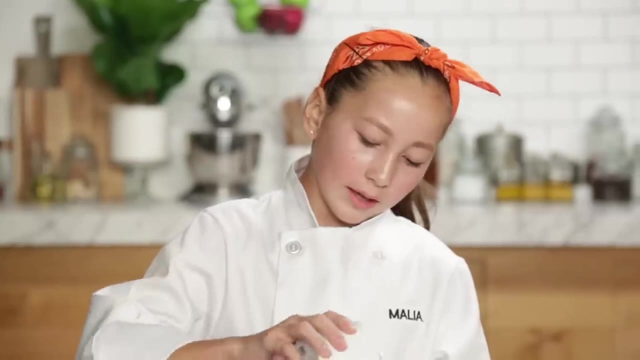 What are you doing? My first step is I'm just taking my ramekins and I'm buttering them and then I'm sprinkling it with some sugar. So how often have you made this souffle before? It's not like my strongest soup, but I feel like, yeah, you've got to live life. 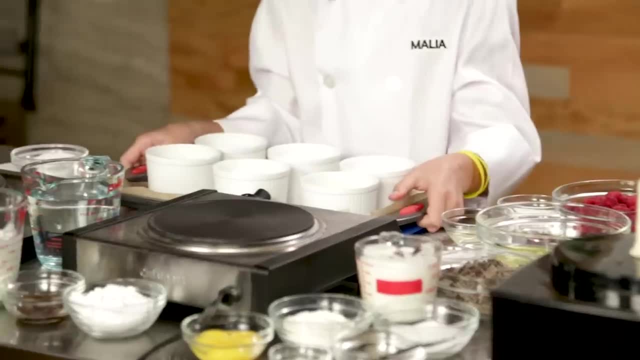 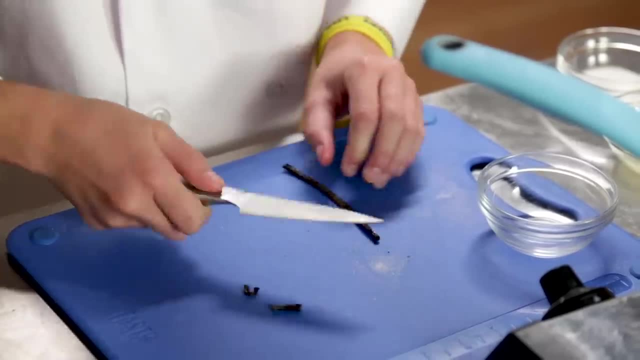 Yes, you've got to live life. Now that these are done, I'm going to go put them in the fridge so they can chill. I think you're feeding me already. I'm taking this vanilla bean and I'm scraping out the vanilla bean pods. 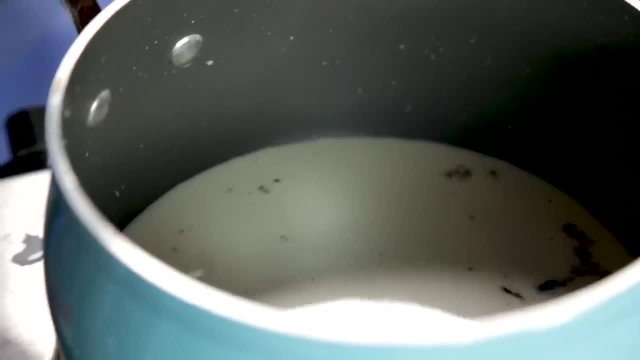 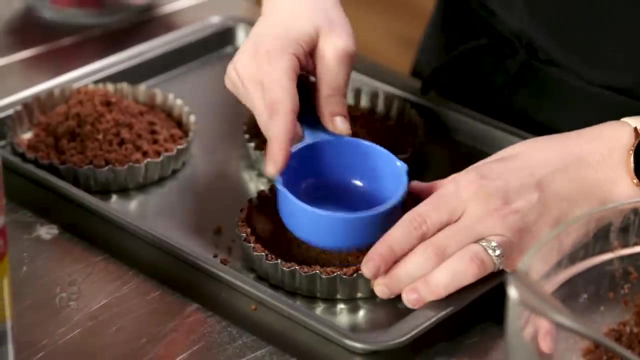 putting this in the pot and then adding my whole milk so that could simmer. So now that my crust is done, I'm going to prepare my tart pans. I just want to make sure that we have the right proportion of crust to- Not too thick, not too thin. you know what I mean. 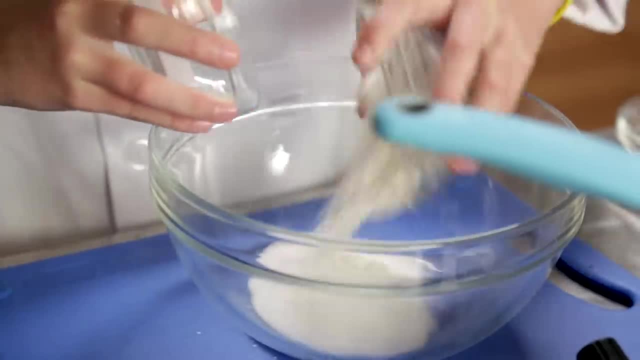 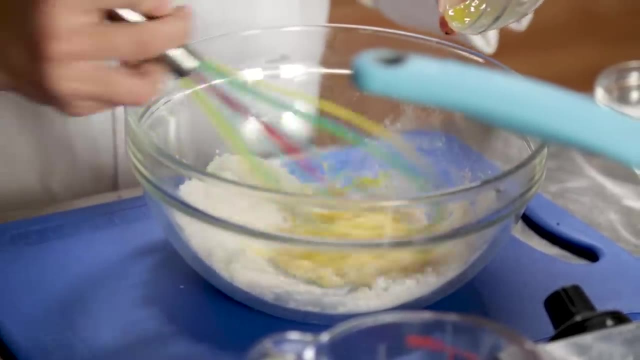 Slow and steady, Slow and steady, I'm dumping my sugar and my flour into a bowl. Then I'm going to add my three egg yolks. After that's done, I'm going to gradually put this in and I'm going to whisk. 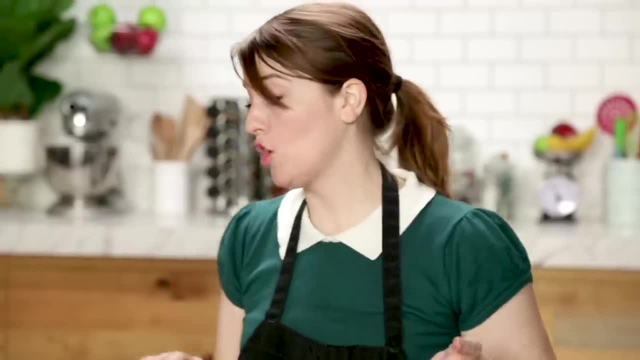 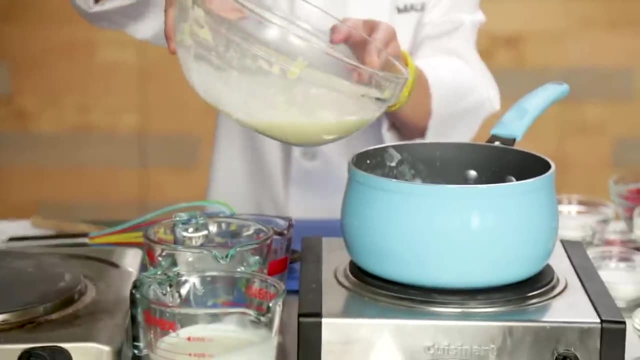 Once you commit- you just got to commit, Good. Well, while you do that, I'm going to go bake these. All right, good luck, Thank you. So now I'm just going to put this back in the pot and I'm going to let it boil for one to two minutes. 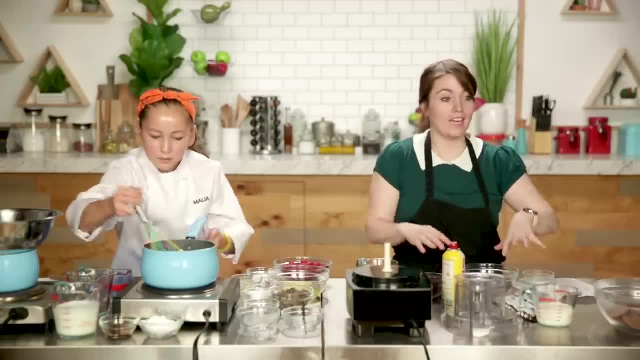 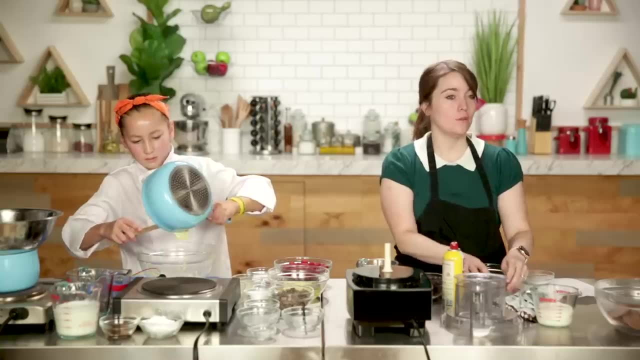 I think Malia's doing awesome. She's got lots of burners going and I'm very impressed. I think that the flavoring and the texture is going to be a winning combination. So now I'm just taking my thick dough out. 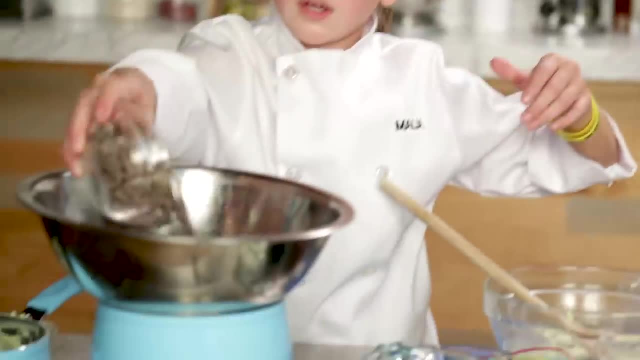 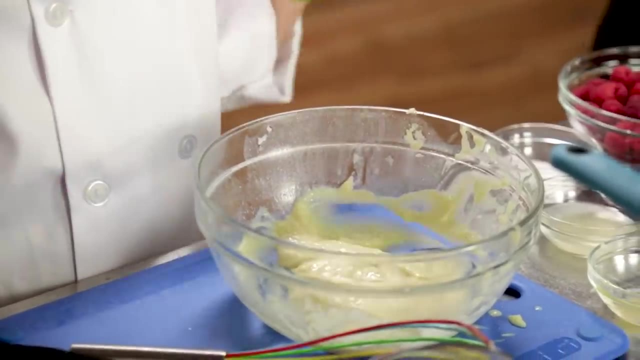 and now I'm just going to add my dough, I'm going to add my dark chocolate into my double boiler and I'm just trying to have this melt as soon as possible, so then I can just put the chocolate into here and then I seal it tightly. 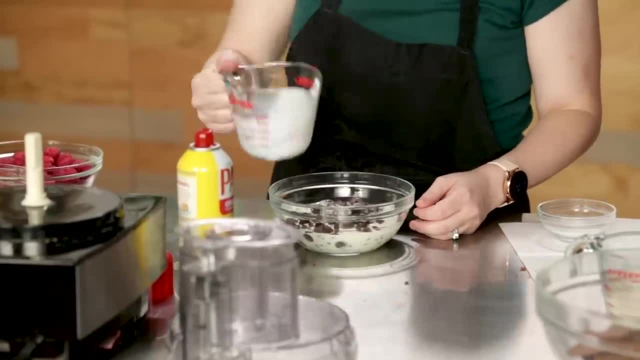 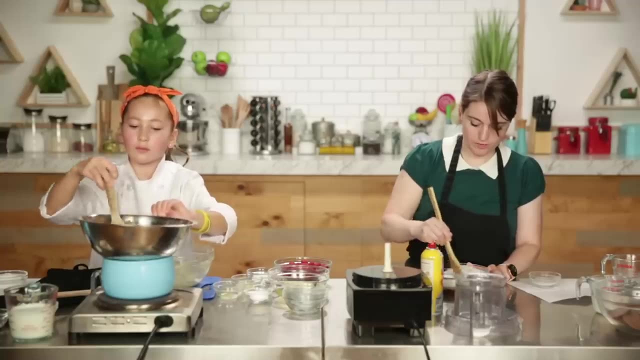 Yeah, it's good. So I'm going to make my ganache now and I'm just going to heat up some heavy cream and put it with some dark chocolate. As you can see, it's really melting, all the chocolate Picking it up here. 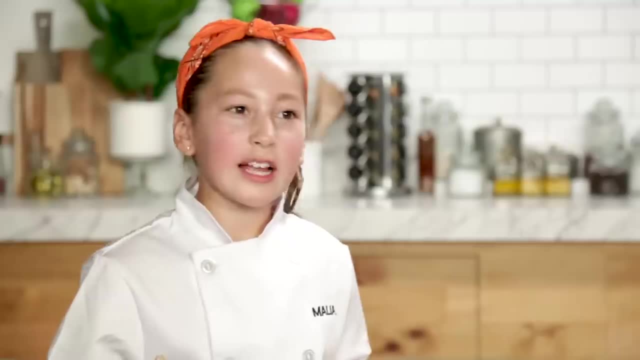 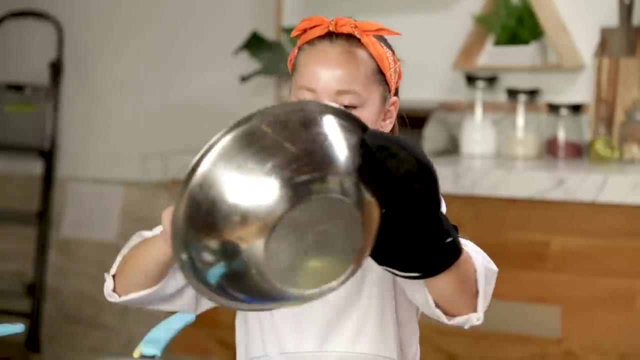 I'm going to go check on my crust and I'll keep coming back. That's awesome As long as Katie's not here. Good, We are just putting this into here and now we're just going to mix. Did you miss me? 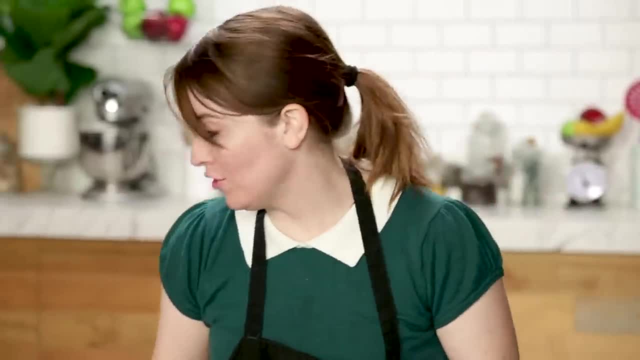 Yes, Yes, Okay. well, my crusts are done. if you wanted to know, Cool, I'm going to pour my ganache now. So, Malia, what do you want to be when you grow up? All right, 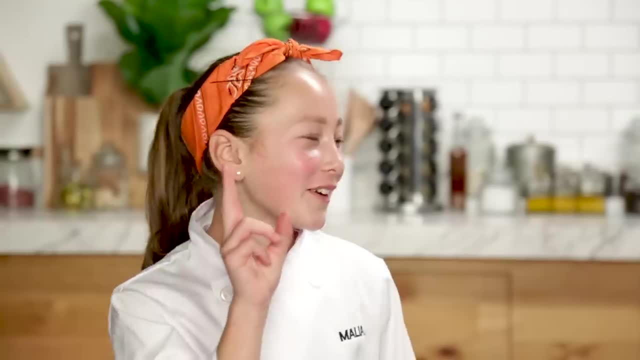 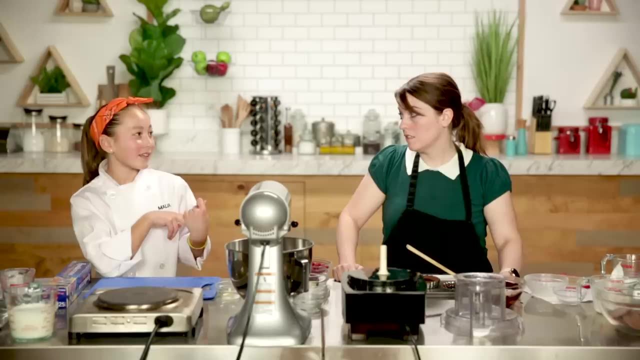 Do tell me Let's dig in A lawyer or a nurse. Wow, Those are so good And I want to be a critical care nurse. That's going to be intense. Yes, That's going to be. Are you ready? 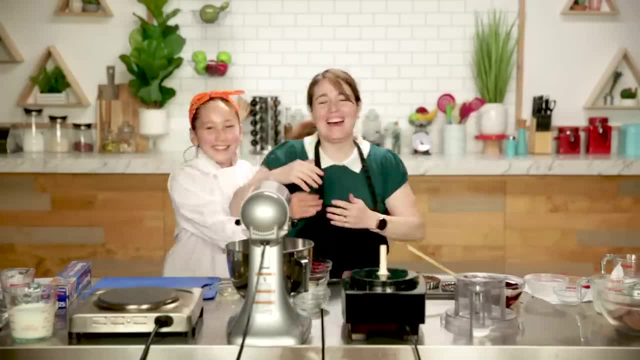 I am ready, Like if I trust. fold right now, you'd catch me. Yes, Okay, I'm ready. No, look. No, you'll be great. if I was in critical care, I would want you at the door, being like hello. 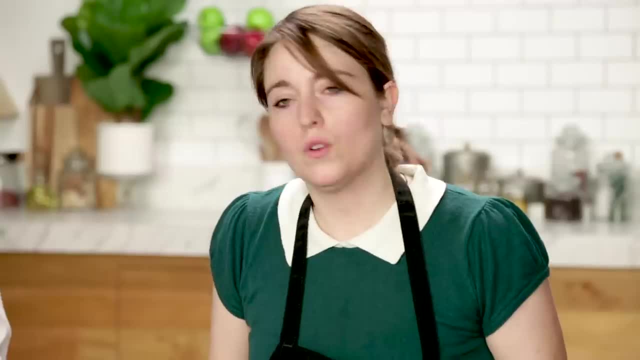 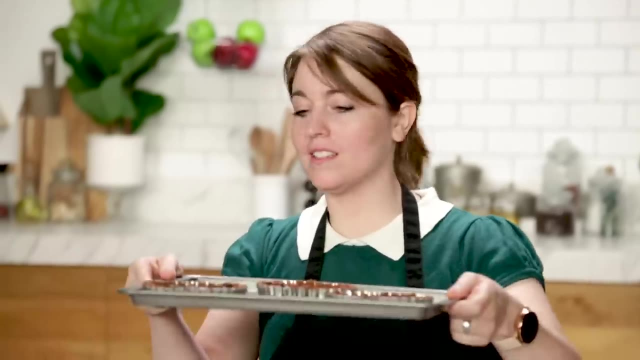 Here's a souffle and a big needle, And a big needle. That's right. You can do it all, Malia. I believe in you. I'm just going to keep producing tasty videos. I'm going to go put this in the fridge. 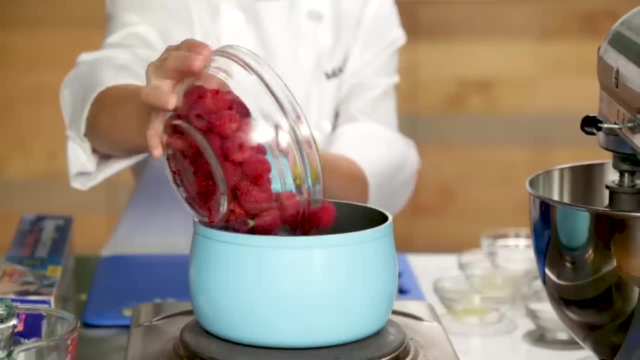 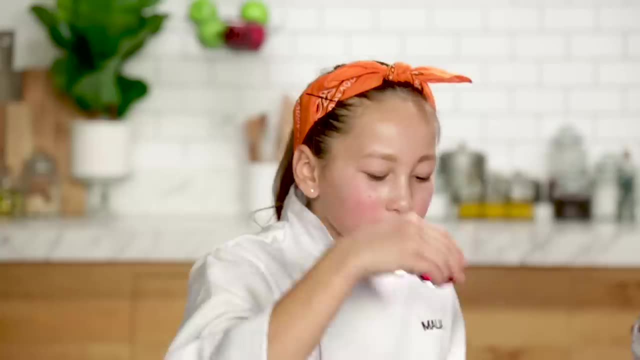 We can even put it in our like strong freezer just to speed this time up. And now just went in my pot. We have the raspberries, sugar and lemon juice And just for a little kick, we are going to add some Chambord. 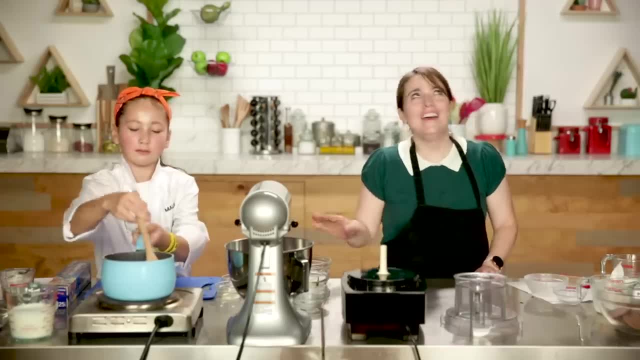 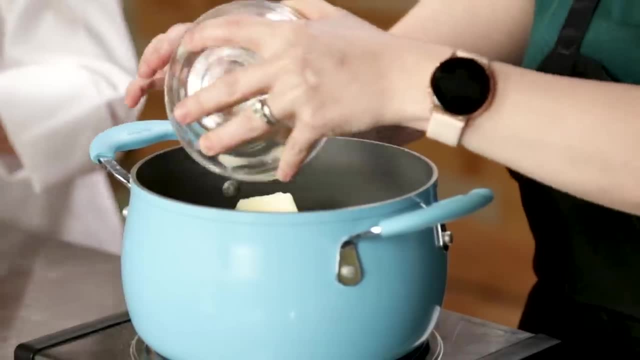 Are you allowed to drink that? That's alcohol, right, It cooks down. OK, I'm going to start making my caramel. It's brown sugar. We're going to do some butter, And when I say some, I mean a lot of butter. 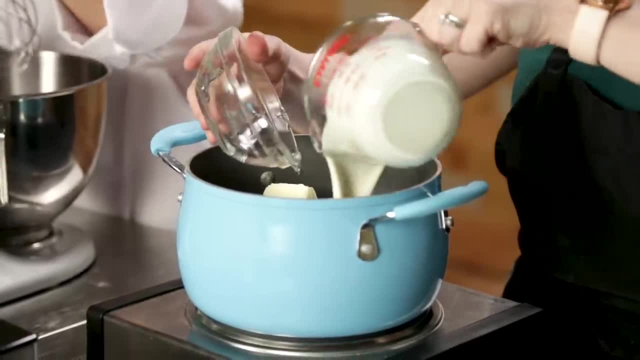 We're going to do some light corn syrup, And then I'm going to add some heavy cream, And then we're going to add some salt. What I am worried about is that this won't set in time for the judging, so It's OK. 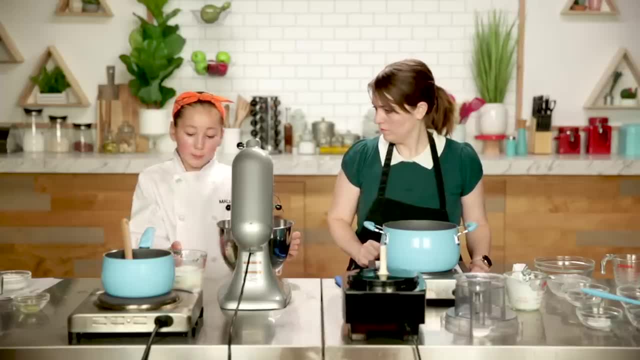 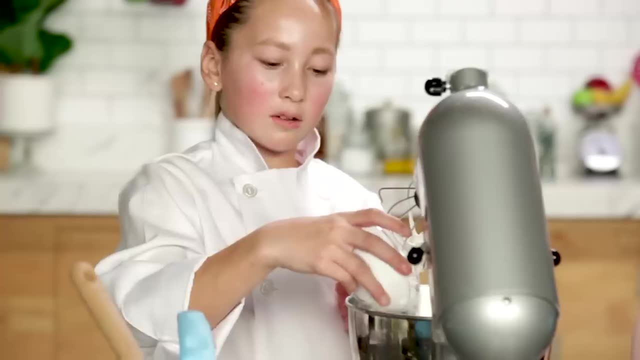 It's OK, Thank you. So you're making whipped cream? Yes, I'm pouring my heavy cream, So it just gets started and fluffy. Then I add my powdered sugar. I'm just going to add it half because I don't want it to like. 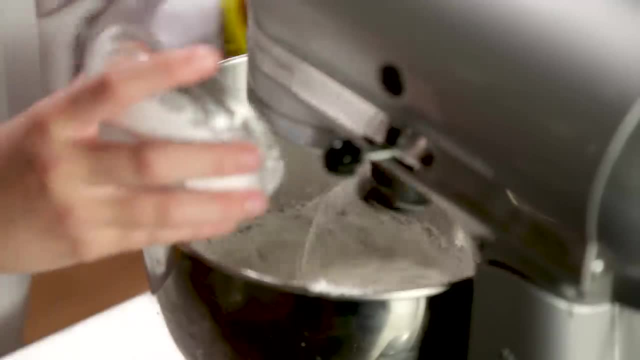 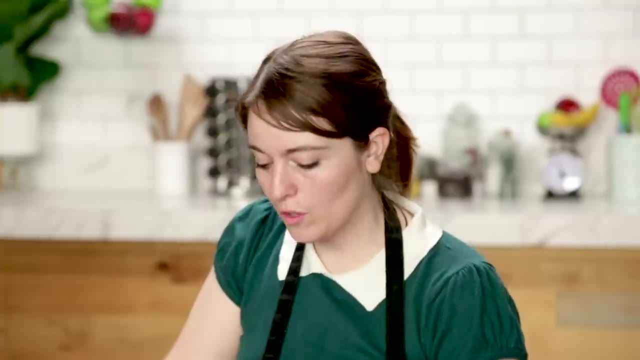 because I've had that happen before. Just add the rest in slowly. So now I'm going to go put this in the fridge. So my caramel's really. it's starting to boil right now And I'm back. Did you miss me? 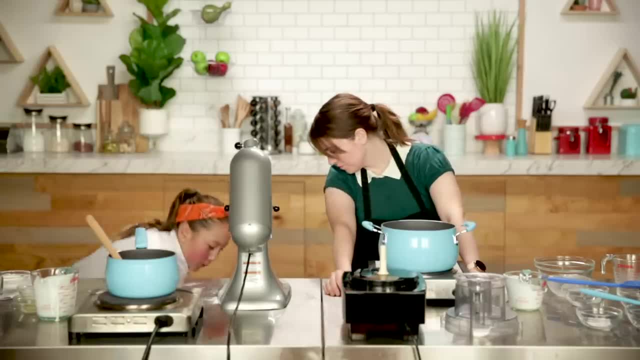 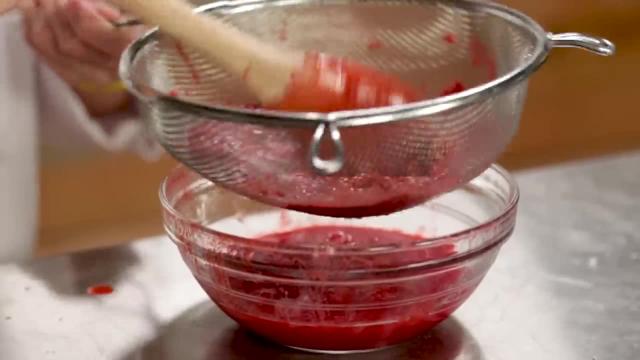 I'm, yes, I mean it. Now I'm just going to grab a bowl and a strainer. Ooh, OK, Because this is like kind of like a compote or like a puree that you're going to like put over it. 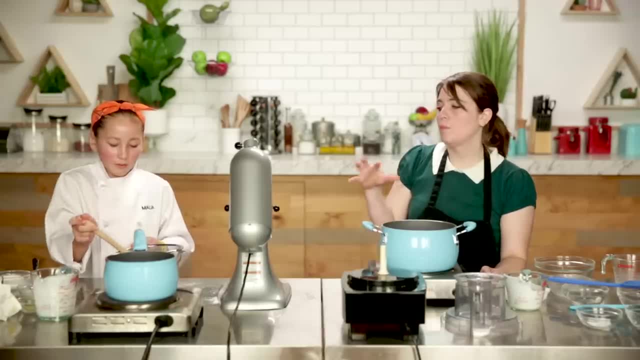 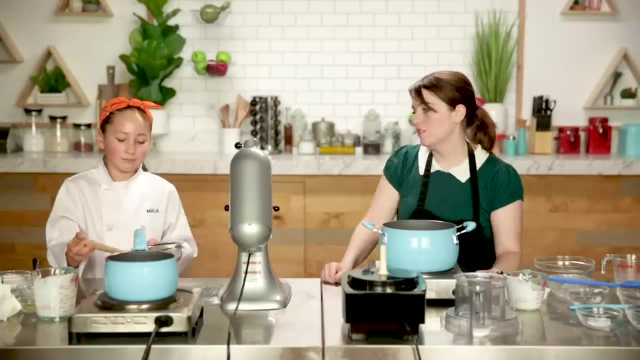 And I guess like this is also a way to make jam. My mom makes really good. we have a pomegranate tree in her when growing up, But I wasn't allowed to eat pomegranates inside the house because they stain everything. 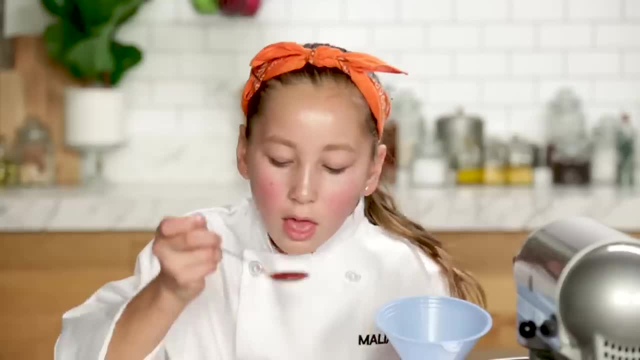 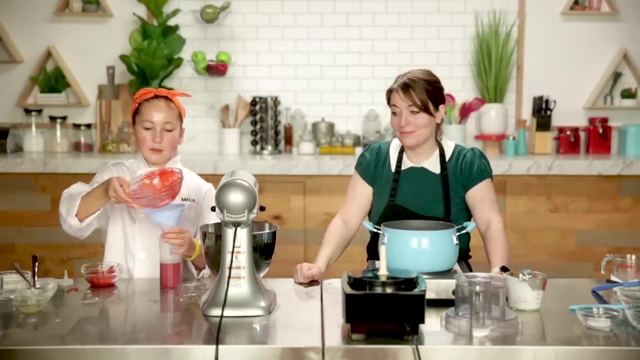 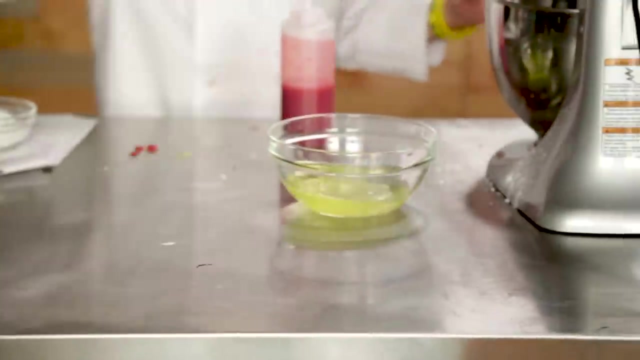 So I had to eat it with a bib outside. Can I try some too? Mmm, mmm, Malia, I'm feeling intimidated. You should be. No, I'm just kidding. Now I'm going to do my egg whites. 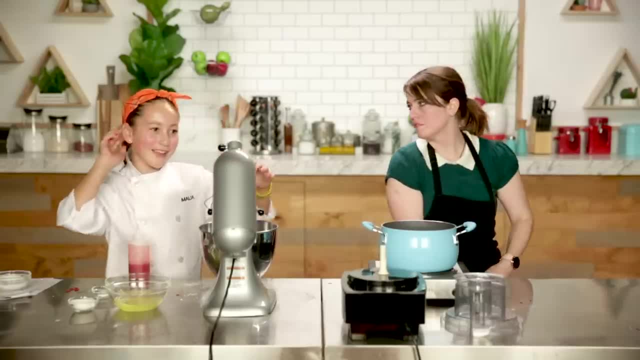 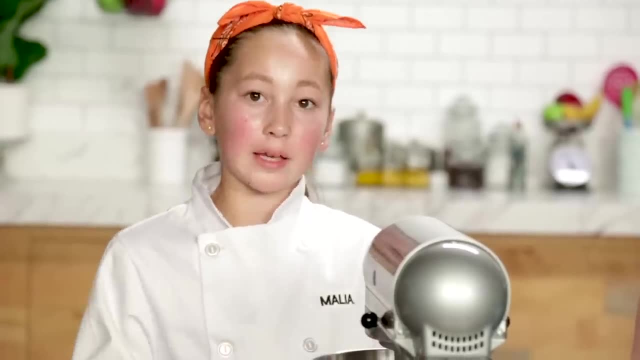 So it's nice and fluffy. Are you doing an accent? right now I'm on a gas side, I was very cold, Are we British? And when it has soft peaks, I'm going to add my fine sugar: Fluff, Fluff. 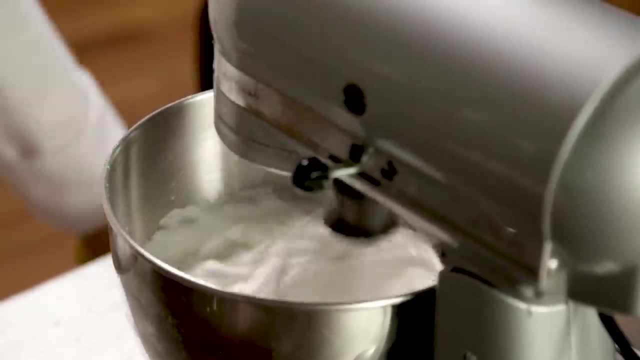 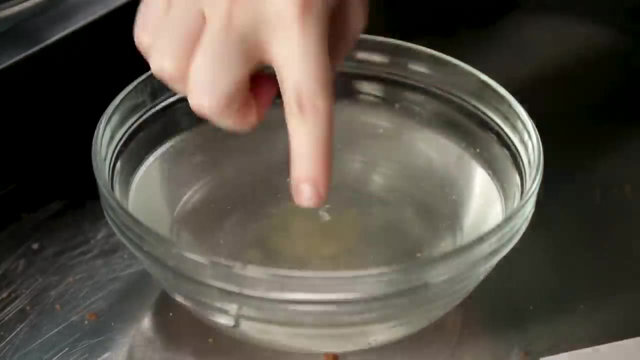 Fluff. Oh, it is getting really fluffy, Yes. So how you can test caramel is you can take some and put it in a cold bowl of water And then you can see if it balls up, And you kind of know if you're close or not. 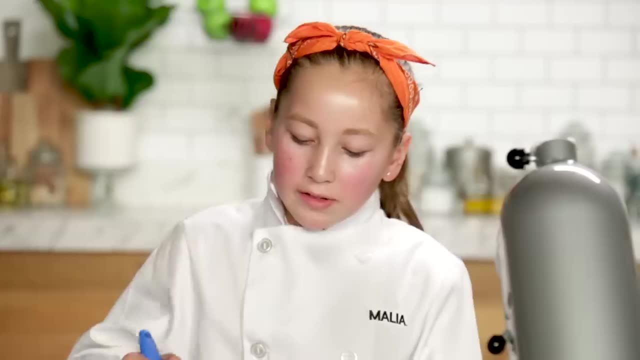 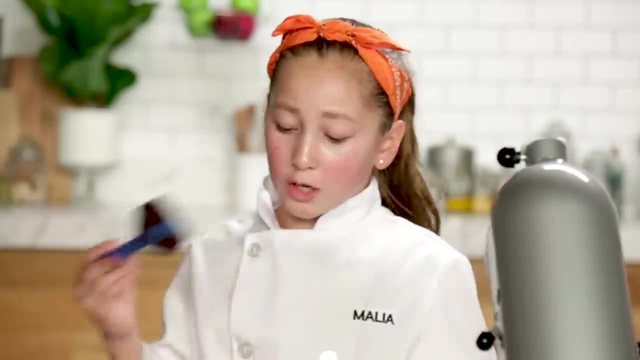 And I am not close, So I just got to wait a few more minutes. Now that this chocolate base is back from the fridge, I'm just going to add my fluffy egg whites. A third of it is going to go in. We're not going to fold this one, because we 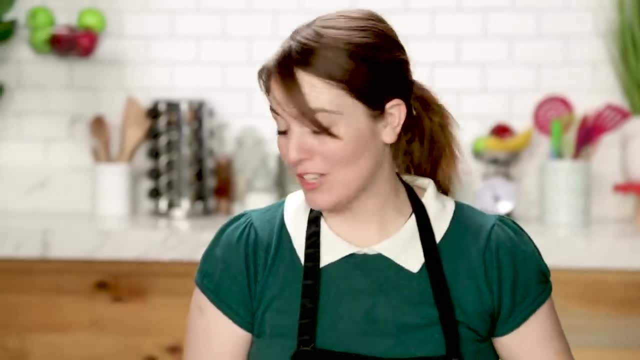 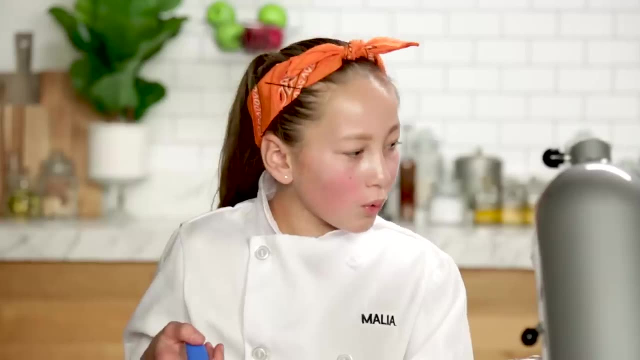 want to get a little bit of texture. I put my ganache in the freezer and it got really hard, But I think that's going to be OK, Because I'm about to put hot caramel on it. So here goes my caramel. Oh god. 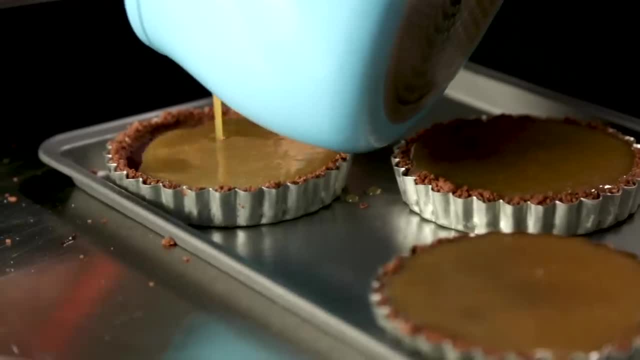 OK, we're just going to slow this one down. OK, I'm going to just now do my sea salt. I got a little excited And now it's a little bit more set. I'm going to do it on this guy. 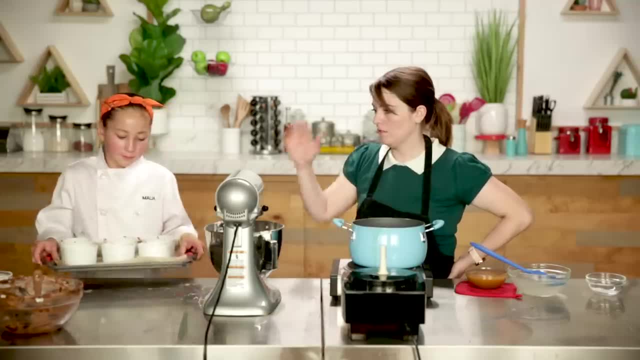 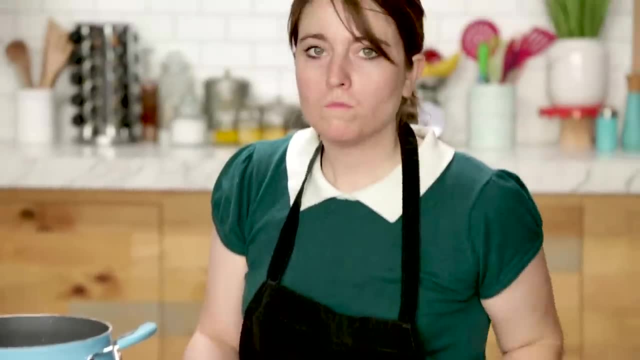 Now all I have to do is go put them in the oven. OK, great, All right, I'll be back. OK, I'm going to hang out and eat some caramel and some cookies, Mm, mm-hmm. So next I'm going to take these tarts out of their pans. 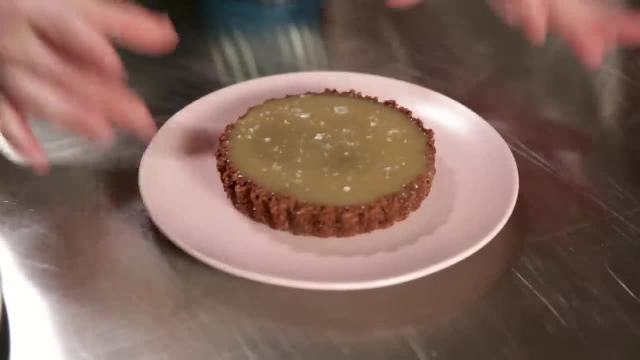 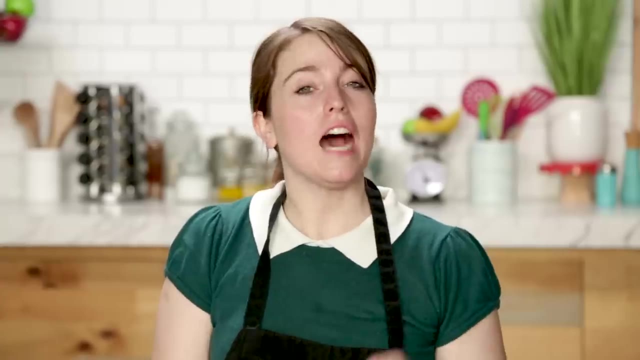 And put them on a plate. I have melted some chocolate And I am using a piping bag just to do like a nice little drizzle across the top. All in all, still feeling pretty good. I still feel like I could win this thing. 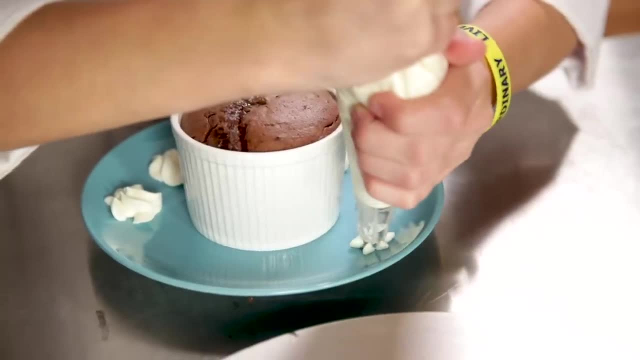 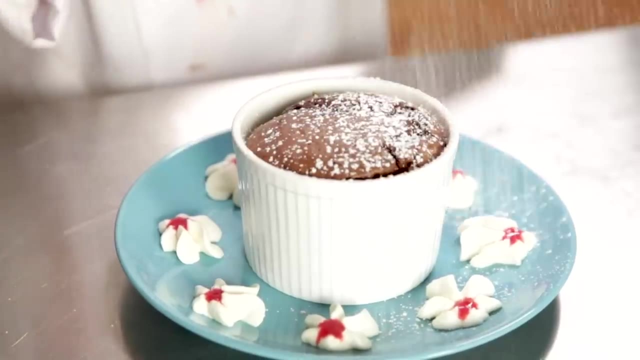 So my soufflés just came out of the oven And I'm just going to put dollops of whipped cream on the outer side of the plate, Drizzle the plate with raspberry coulis, Take my powdered sugar And I'm just going to sift it, sift it, sift it. 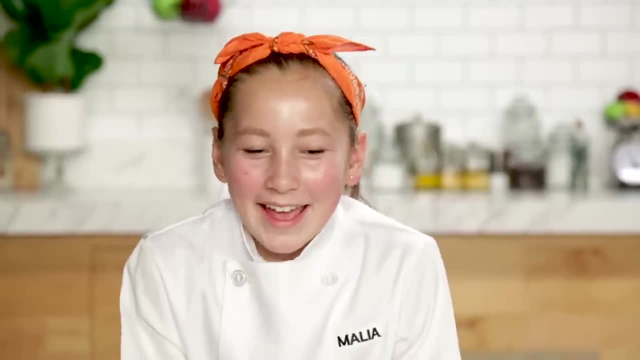 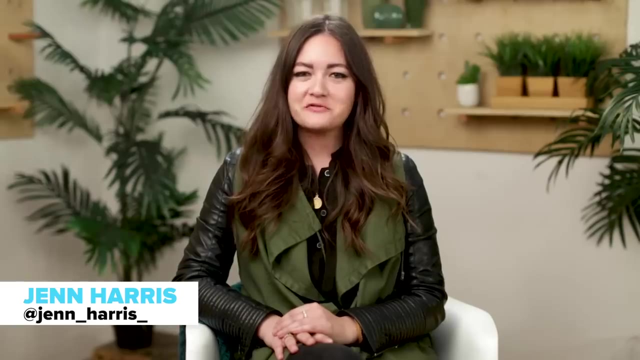 Then a raspberry on top. I do think I'm going to win. I wish her the best of luck, But later, skater. I'm Jen Harris And I'm a senior food writer for the Los Angeles Times. Today, I'm going to be judging the dishes. 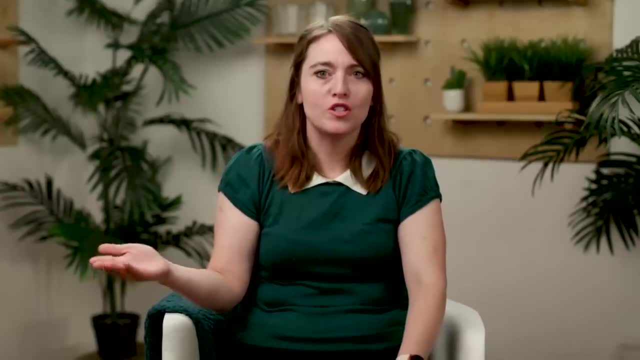 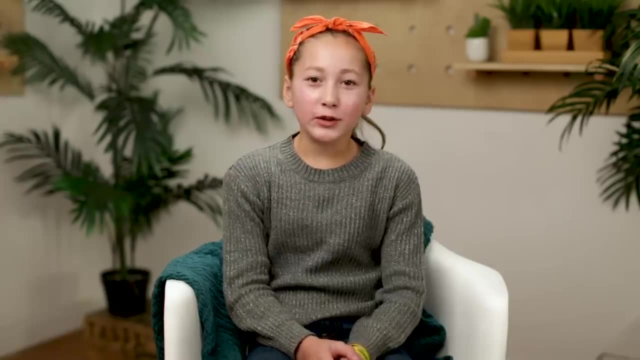 that Katie and Malia made. Nobody told me Jen Harris was going to be judging this competition. She's tried all the food. She knows all the chefs. She's written about tons of restaurants. I think Jen will really like my food because I try to cook for my culture and my heart. 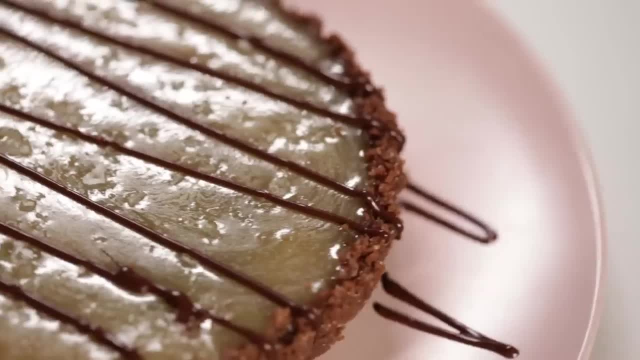 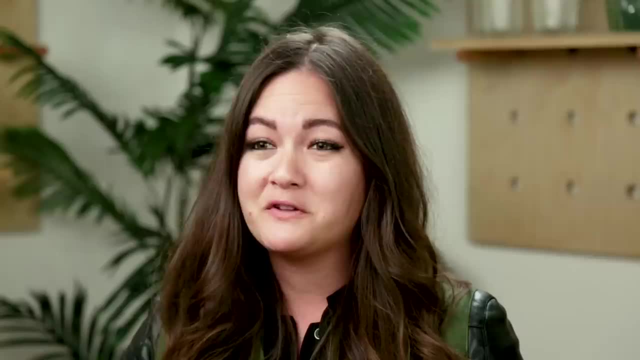 For me, what makes a good chocolate dessert is something craveable. It has to have like good chocolate flavor. But I also like a little bit of salt, a little bit of sour, something to balance out all that heavy chocolate. I'm going to be looking at plating. 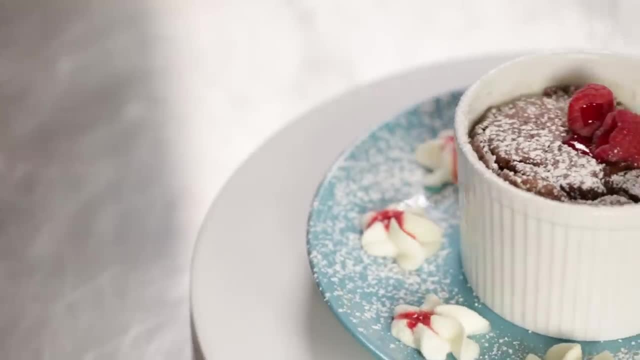 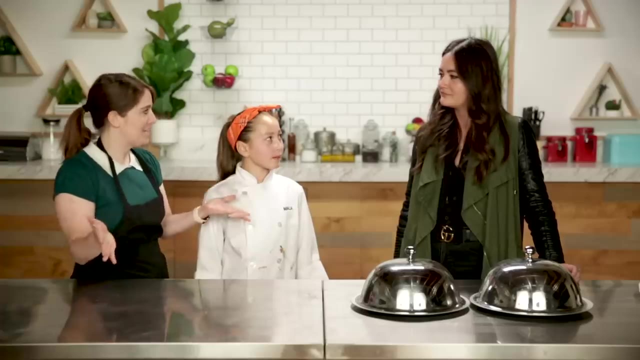 Does it look like something that would be at a fancy dinner party? Does it look like something I'd want to pay a good amount of money for? I really have no idea who's going to win. Hey, Jen, Thank you for coming to judge today. 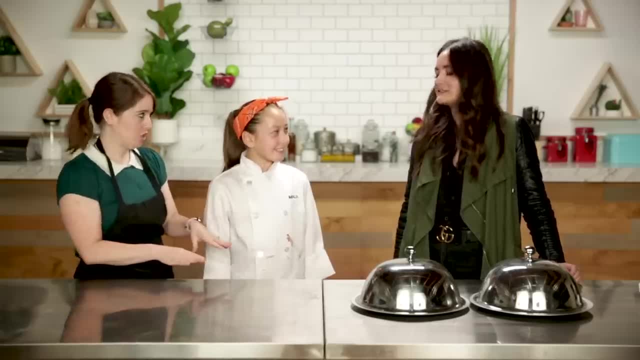 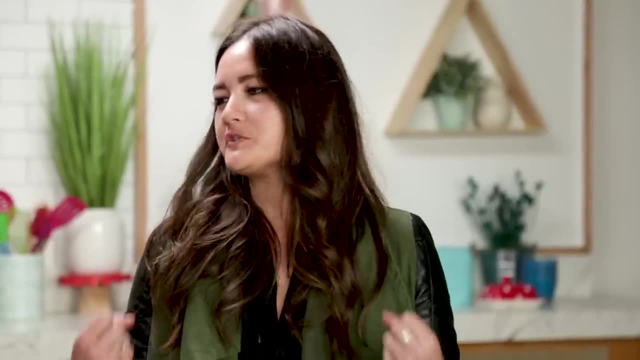 Thanks for having me. We're not going to tell you who made what dish. Are you excited? Yes, I'm a little excited. I'm a little nervous, Me too, But we're fine, It's calm, Don't be nervous. 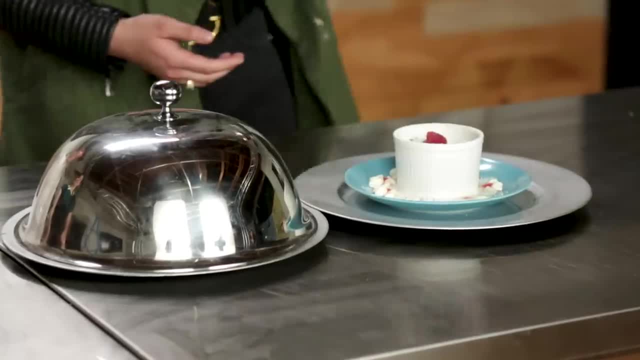 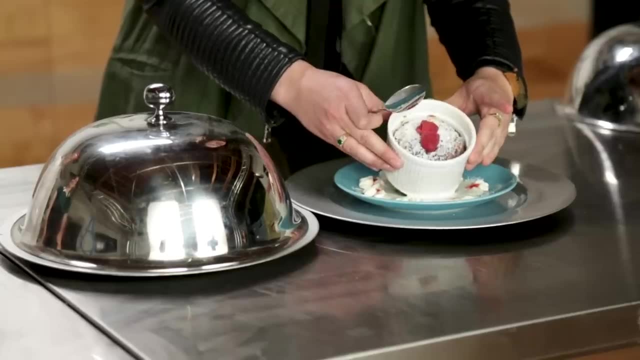 I'm just super tough. I'm going to start with this one. That is beautiful. I already like the plating. See, it's supposed to be a souffle. It has fallen a little bit. It is not exactly as high as I would like it. 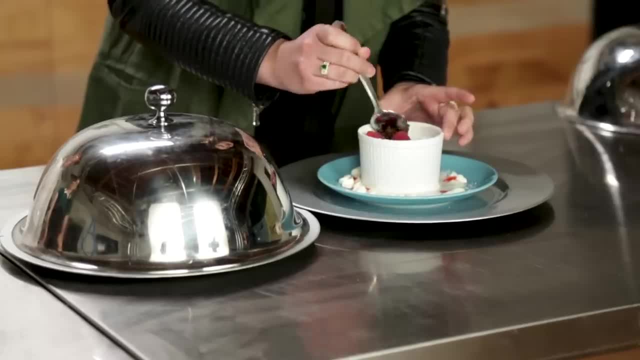 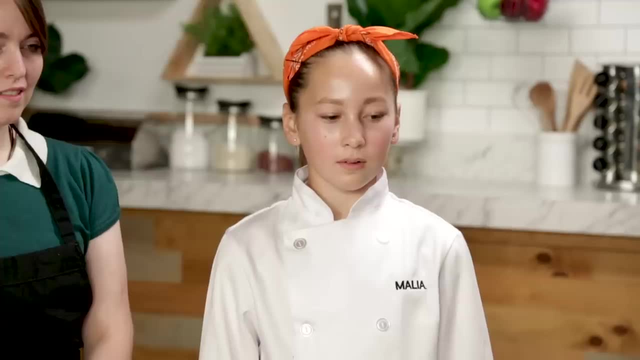 Still warm, though. Texture is really good. It's super light, nice and cakey. There's like a little bit of crust across the top. Let me get a little bit of this sauce on there. This souffle is pretty fancy. 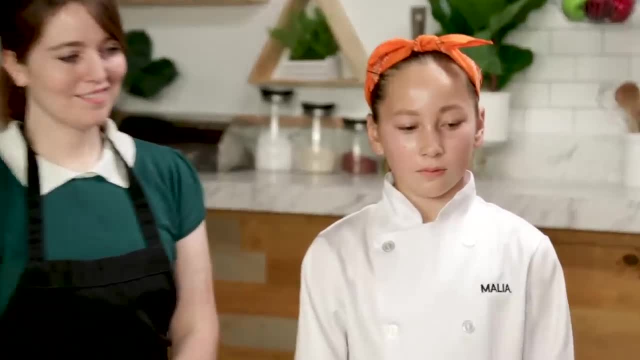 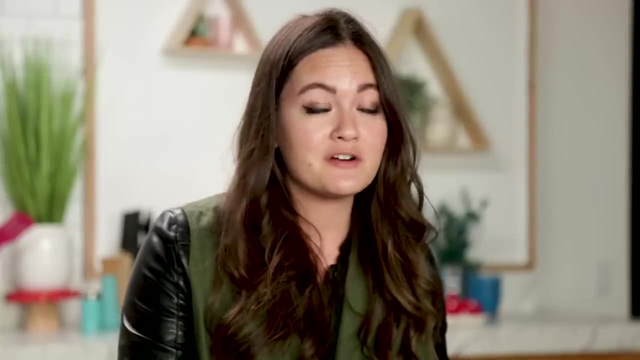 I feel like if I went to a restaurant, and I went to a five-star restaurant and I ordered this for dessert, I'd be really happy. A little disappointed that the souffle fell, but in terms of flavor and texture, the chocolate flavor is like a really nice punch of chocolate. 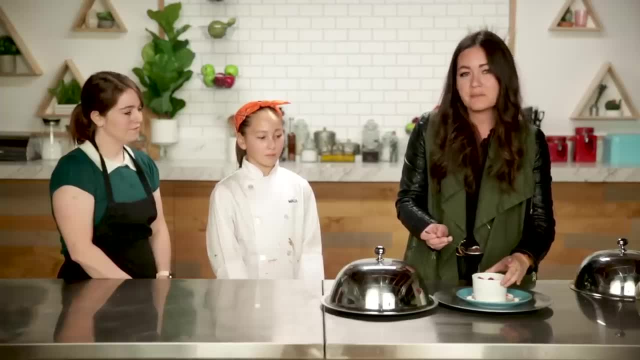 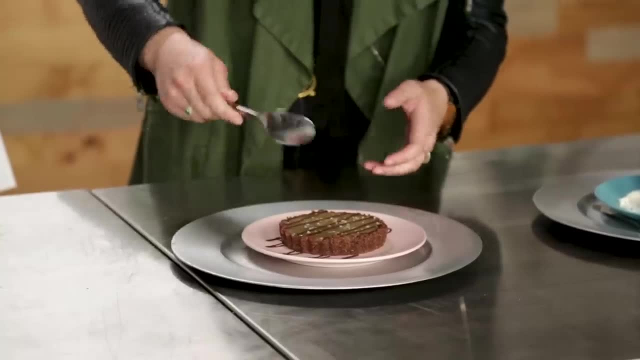 balanced out with that like cool raspberry coulis. Very impressed with this Dessert number two. Oh So kudos on the plating. I like that little drizzle of chocolate on there. I think it is a caramel tart of sorts. 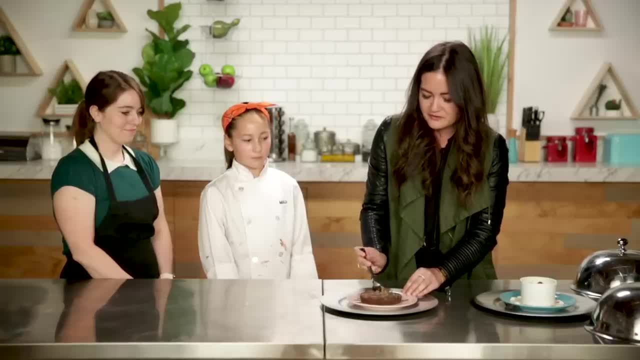 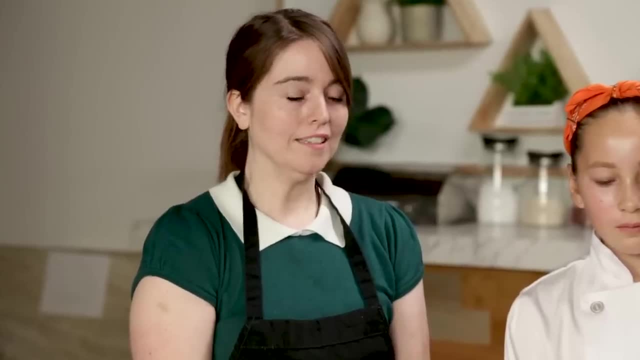 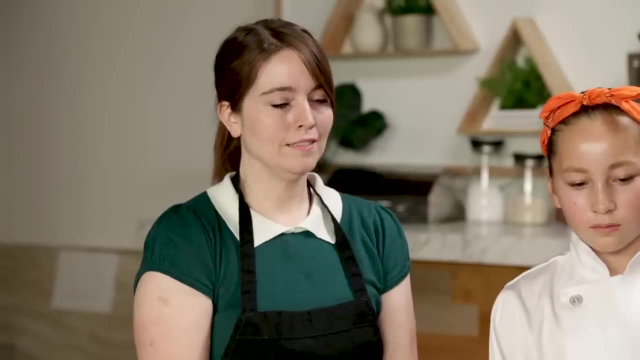 I like the crispy Crunch of the crust. already This is also very good. Good level of sweetness. I love the flake sea salt on top. You very much taste the caramel, so you can't really taste the chocolate. It's getting a little lost. 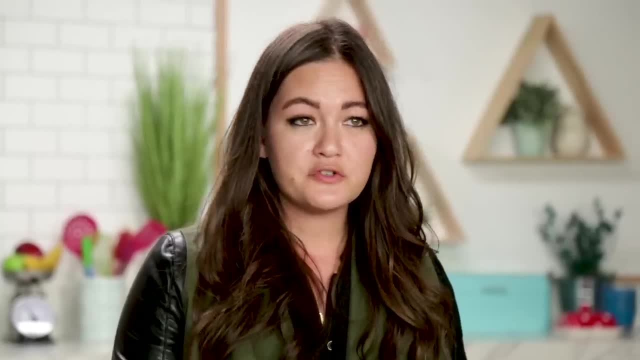 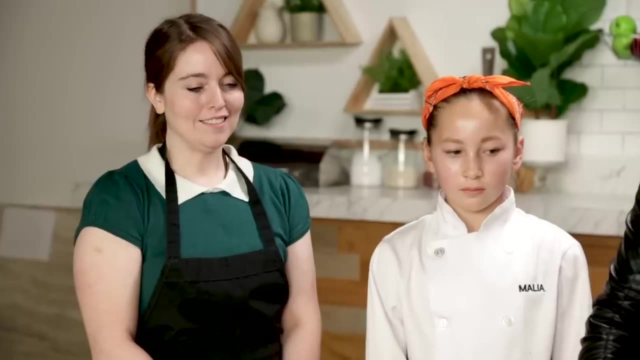 but I would definitely eat this entire thing still. Both of these desserts were super fancy. I would be happy with either of them, but I was told I have to pick a winner, so I'm gonna pick one, And the winner is the chocolate souffle. 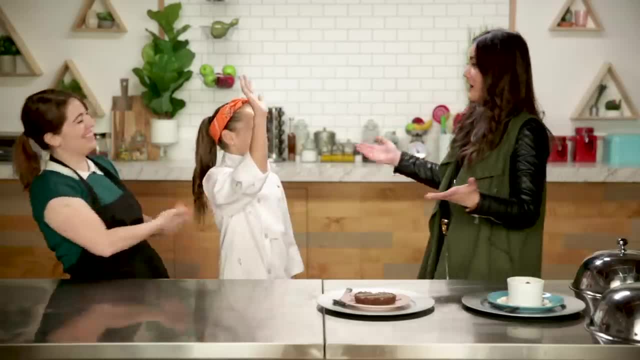 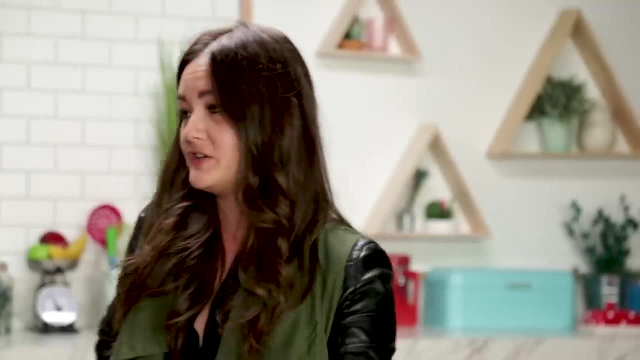 Whoo, Who is this? The chocolate souffle? Oh my gosh. Good job, Thank you. I had faith in you, Thank you, Thank you. Oh, I'm fine, Yours was very good too. No, no, thank you. 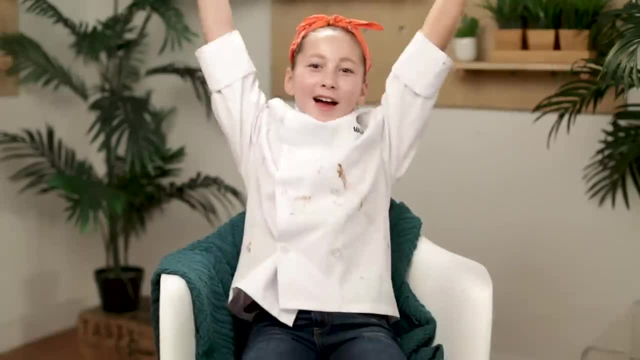 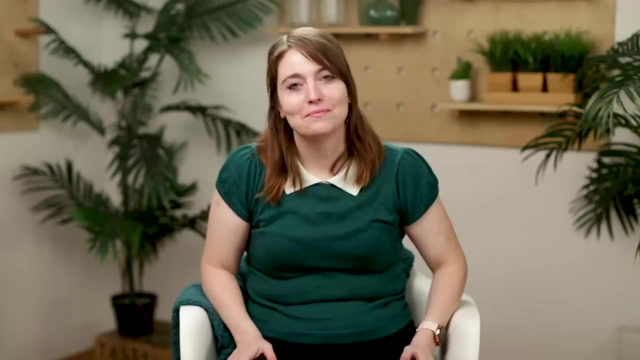 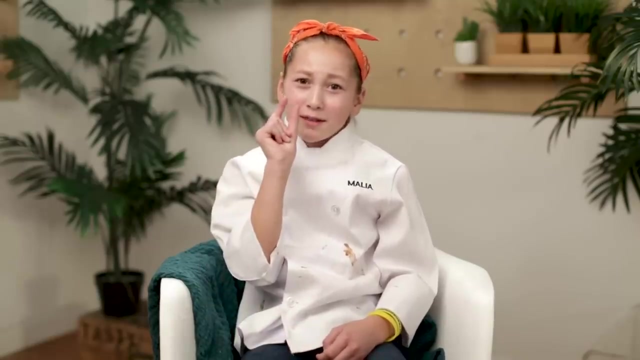 But this is the clear winner. Oh my God, I won. Whoo, I lost. It's okay. Winning is not everything. I'm like pretty sad. I think Jen made the right choice. My advice for Katie is: a little caramel goes a long way. 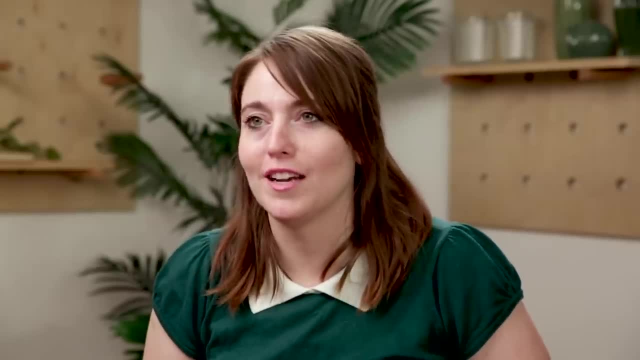 Today I learned that like losing can still be fun, because I had such a fun time cooking with Malia- Like she's just so cool and I still feel good about my dish, so I just feel like I've learned. 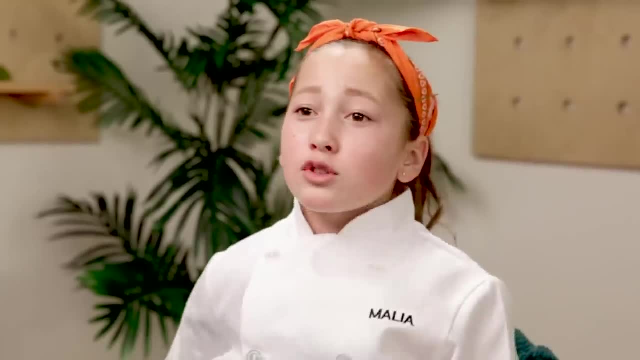 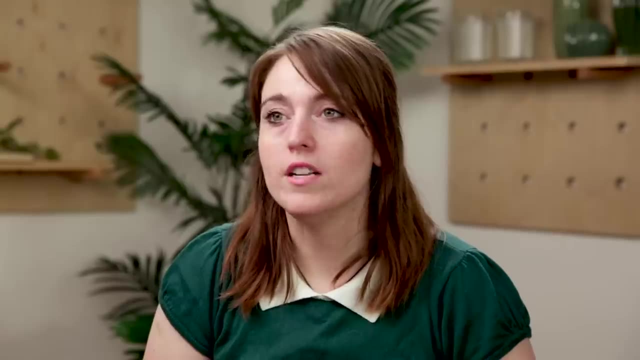 to have a more positive attitude. I love this day. It was super fun. I got to meet Katie and I feel like I'm accomplished. I would definitely rematch Malia just because I could like hang out with her more. 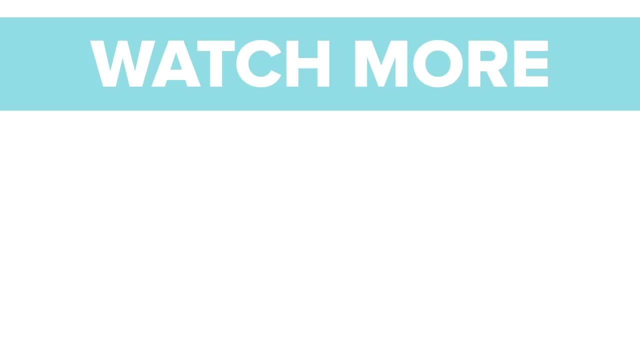 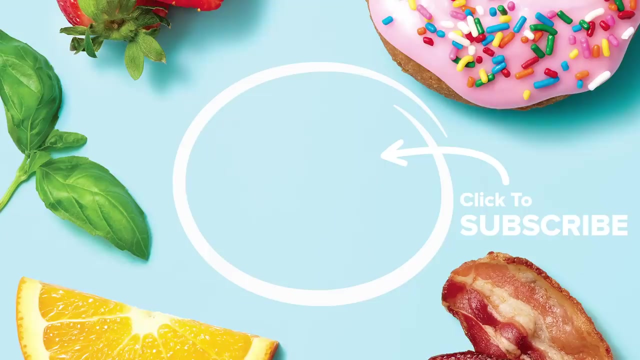 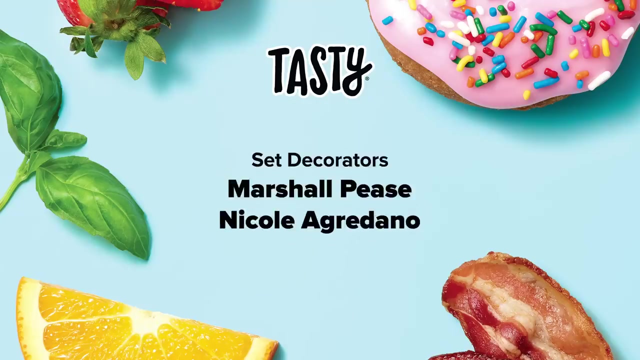 because I really like hanging out with Malia, but also because I want to win. Really, I'm so glad I did. Thank you guys so much. It's been so much fun. Thank you, Thank you guys, Thank you guys. We'll see you next time. Bye, Bye, Bye.